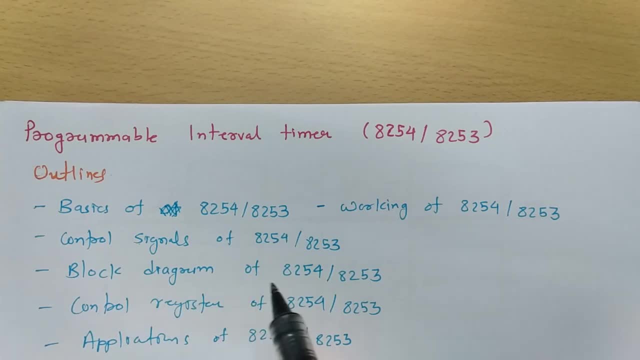 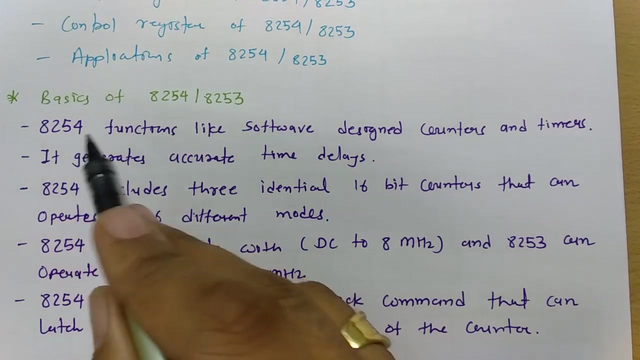 control signals of 8254, block diagram of 8254, control registers of 8254 and applications of 8254.. So these are my session outlines. Let us begin this session with first point, that is, basics of 8254.. Now see 8254. functions like software design, counter or timers, So 8254. 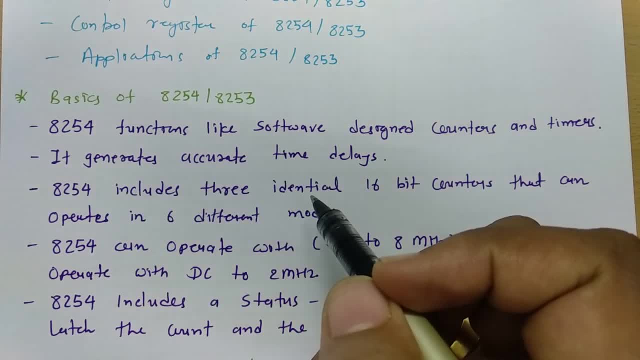 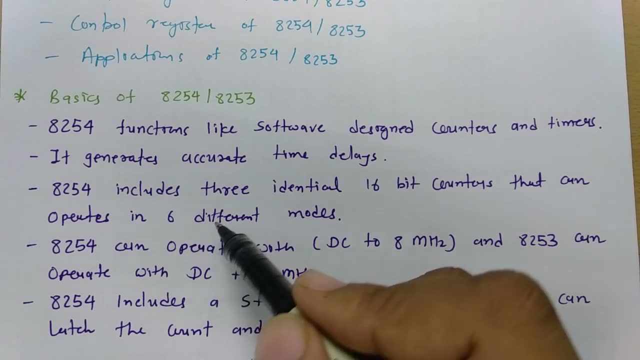 that is been working like software designed counter or timer. It generates accurate time delays, It has 16 bit counters and that can operate in six different modes. So I'll explain all three timers or counters that is there in 8254 and how many modes that is there, how to select those modes. 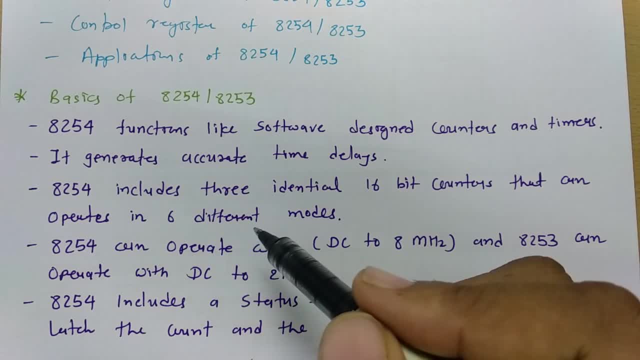 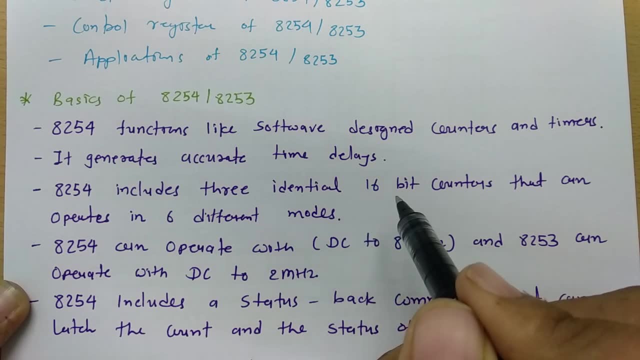 Also all those things that we will see in control register. explanation of 8254.. So basically, 8254 is having three different, identical 16 bit counters and that is functioning in six different modes. 8254 can operate in DC to 8 gigahertz frequency, while 8253 that can operate. 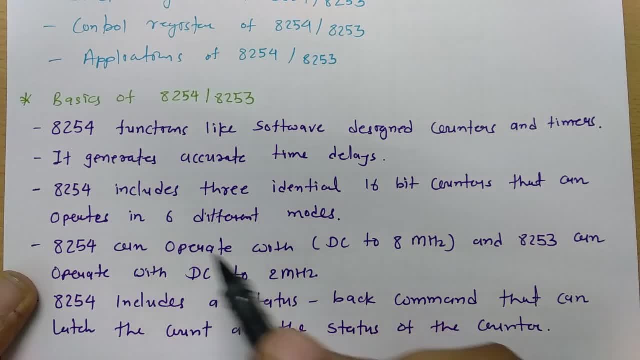 with DC to 2 megahertz of frequency. So 8254, that is advanced version of 8253.. Initially 8253 was there which was working with DC to 2 megahertz of frequency and then after advanced version of that timer, that has been made. 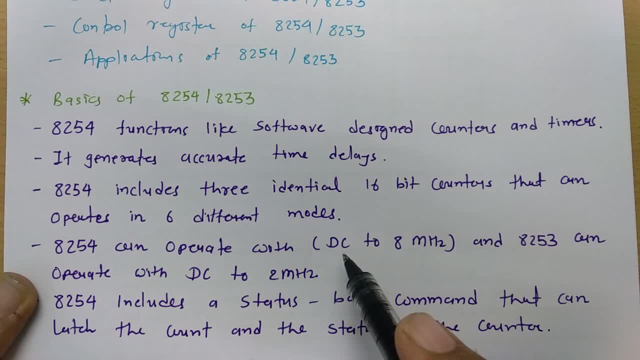 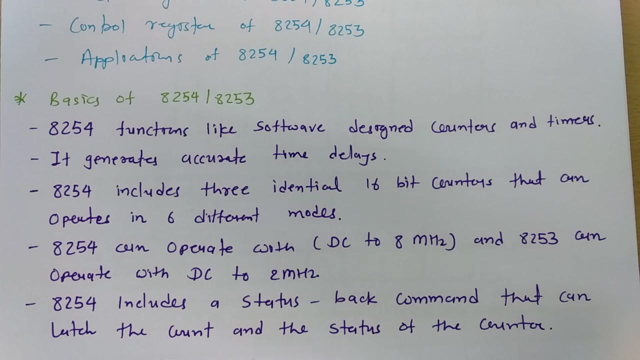 It is having operation frequency from DC to 8 megahertz. that is there with 8254.. 8254 includes status back command and that can latch count and the status of counter. So that status back command that is not there with 8253, which can latch count and the status of counter. So this new feature. 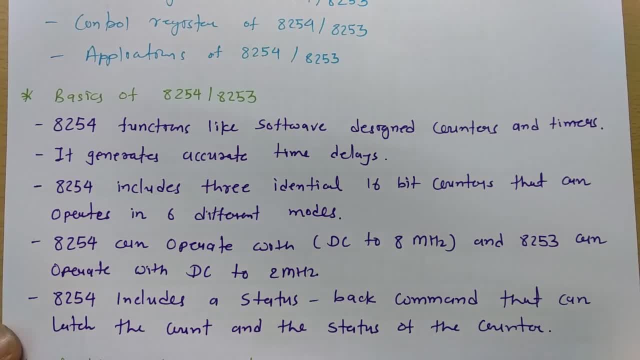 that is there with 8254, which is not available with 8253.. Now let us have a basic understanding for 8254, which explains how it functions. So, as I have told, 8254 that is 16 bit counters and there are basically three identical counters, which is there. 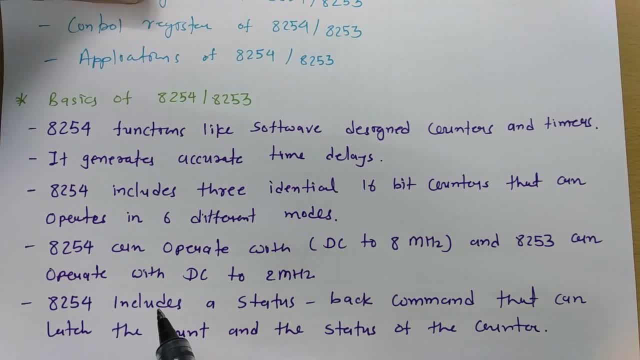 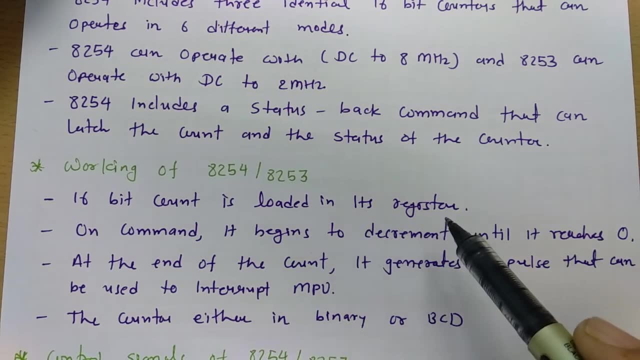 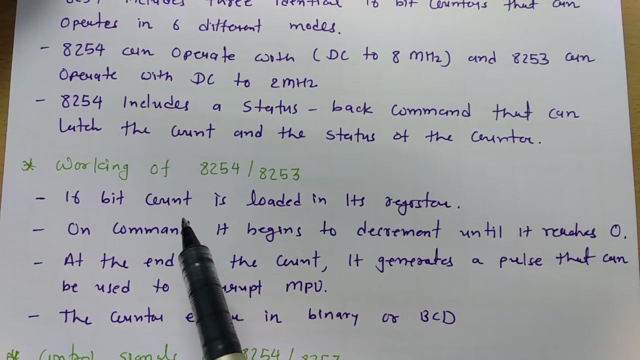 with 8254.. So how those counters are working. let us see that. So 16 bit count is loaded in its register first. So once you load 16 bit count on giving command, it is beginning to count and to count it it will decrement until it reaches to zero. So on, initially we need to load 16 bit count in register and then 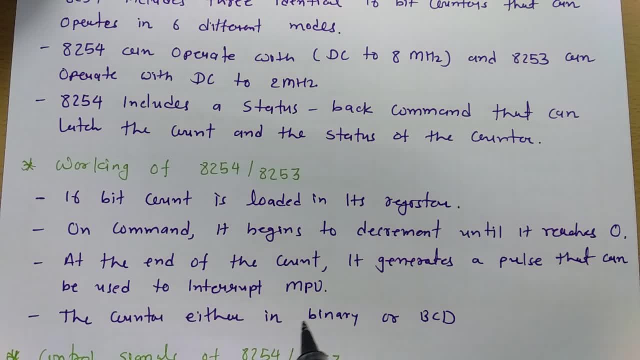 based on command which is given to it. it will start to decrement one by one until it reaches to zero. At the end of count it generates pulse And that can be used to interrupt microprocessor. So at the end of count it generates pulse which is 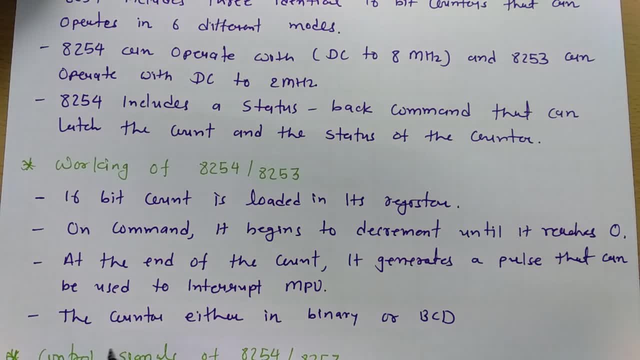 being utilized to interrupt microprocessor. The counter either in binary or BCD and how to select binary or BCD count. that is what I will explain in control register. So basically 8254, that is having three different counters. All three counters are made up of 16 bit. 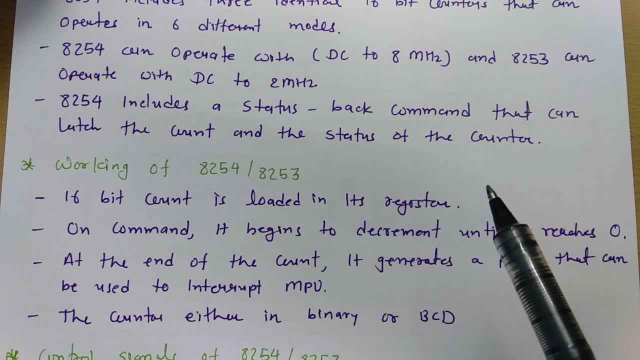 That is functioning in six different modes. That count can be done either in binary or in BCD. First we need to load count into register and, based on command given to 8254, it will begin to count and it will start to decrement that counter until it reaches to zero. 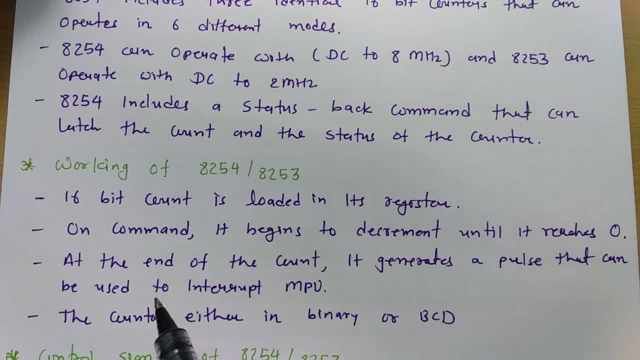 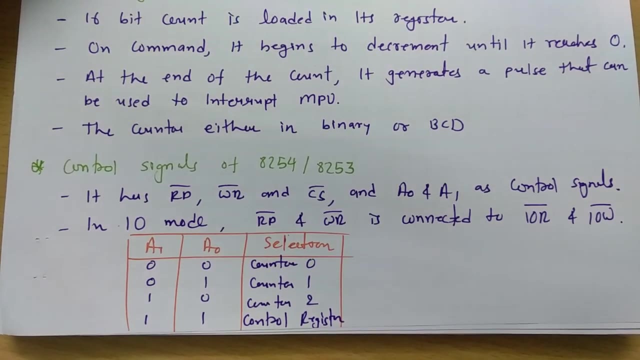 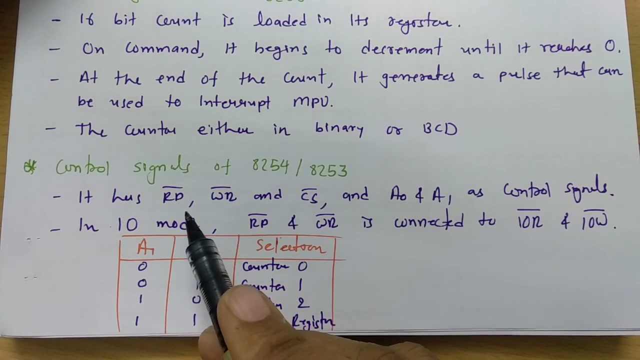 Once it reaches to zero, it will give interrupt to microprocessor. So this is how 8254 is functioning. Now let us see how many control signals which is there with 8254.. So in 8254 there are basically five different control signals, which is most important. 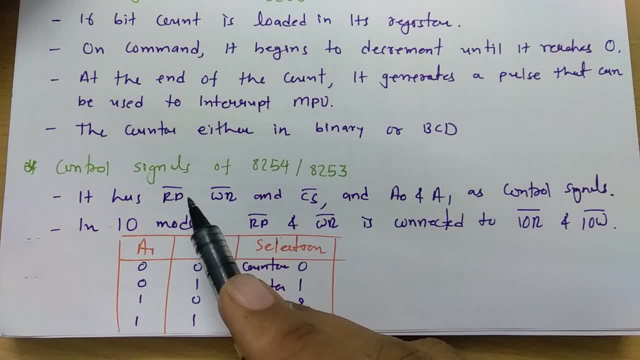 Read bar, write bar, chip select and A0A1.. Read bar: signal that is being given by microprocessor to read the data. Write bar: that is to write the data, And chip select: that is to select the chip A0 and A1.. 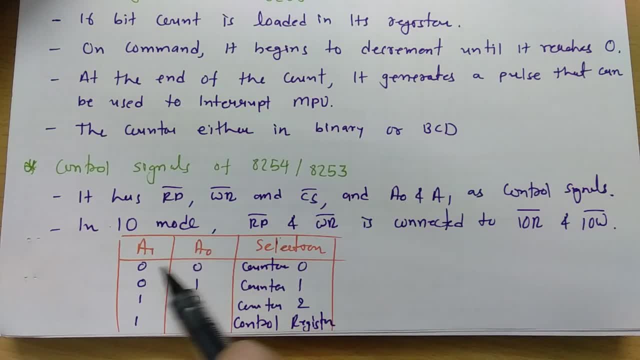 That is selecting counter. If A0A1, that is, 00, that is counter 0.. If it is 01, that will select counter 1.. If it is 10, it will select counter 2.. And if it is 11, it will select control register. 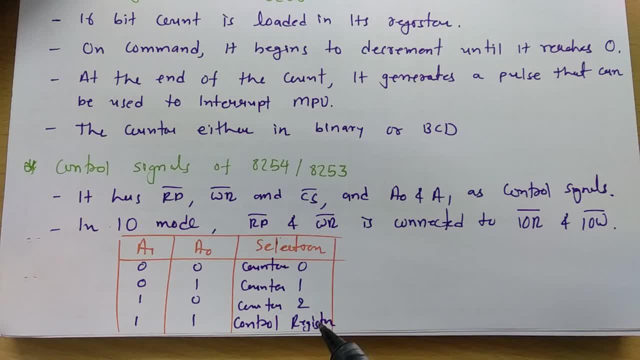 So by selecting control register we can set mode of operation And which type of counter. that is there with a command Likeregaux. So that's it. So the way you say, is phone, WhatsApp or James stand 8254 that we can justify. so first of all we should know how we can select counters and 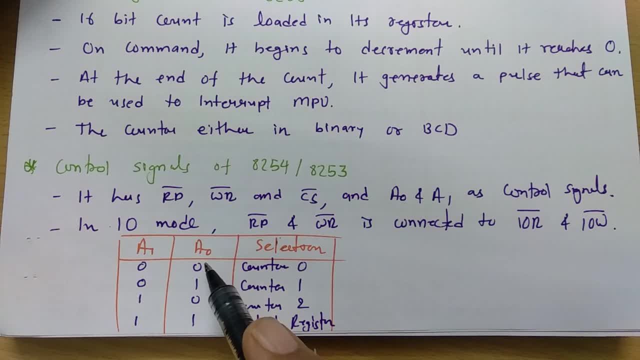 control register. by having a0 and a1 terminal, we can select counter and control register. if it is 0- 0, we will be selecting counter 0. if it is 0- 1, we will be selecting counter 1. if it is 1- 0 we. 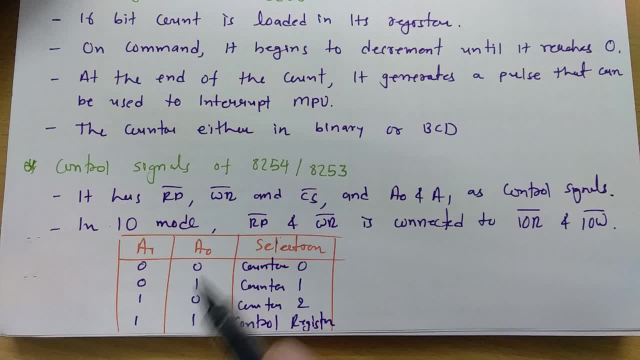 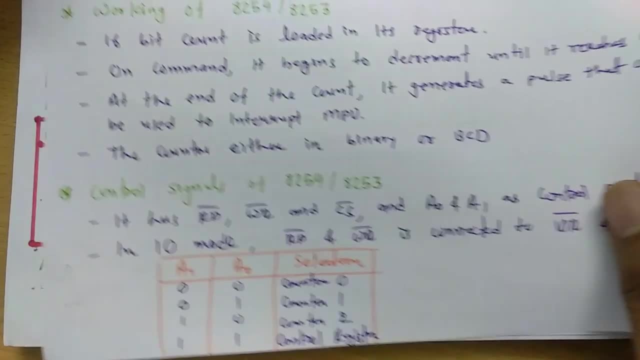 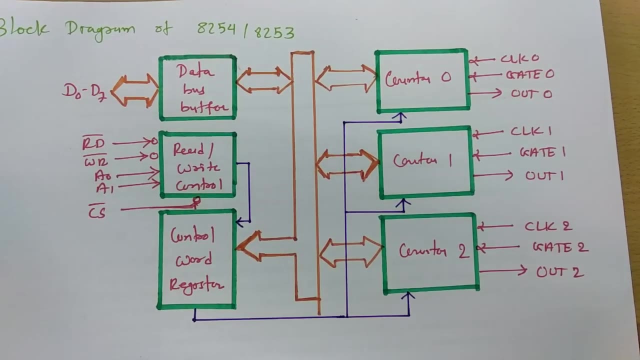 will be selecting counter 2, and if a1 and a0, that is 1, 1, then we will be selecting control register. so let us see first of all what is the block diagram of it and then we will see how control register is operating. so see, in block diagram, as i have told you, there are five control. 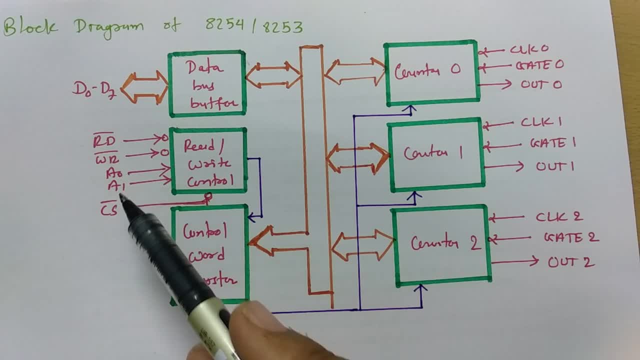 signals: read bar, write bar: a0, a1 and cheap select. cheap select is to select this. it 8254. cheap read bar: that is the signal given by microprocessor to read the status. write bar is to write the status a0 and a1. that is to select counter. if this a0, a1, that is 0, 0. 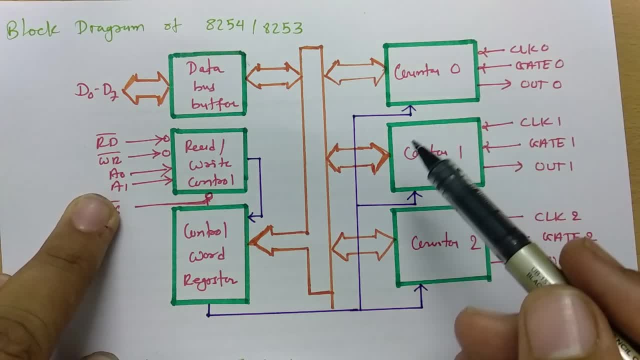 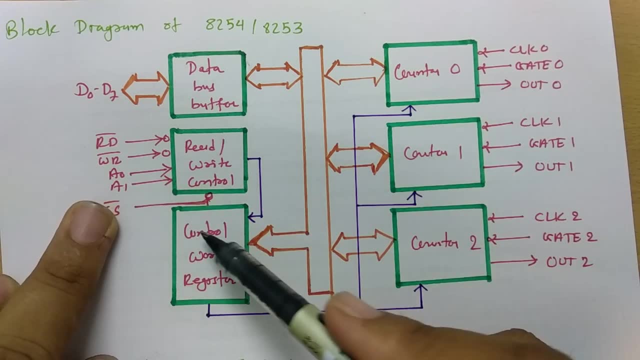 this counter 0 will get selected. if it is 0- 1, it will select counter 1. if it is 1- 0, it will select counter 2, and if it is 1- 1, then it will select control register. so it will select this register. 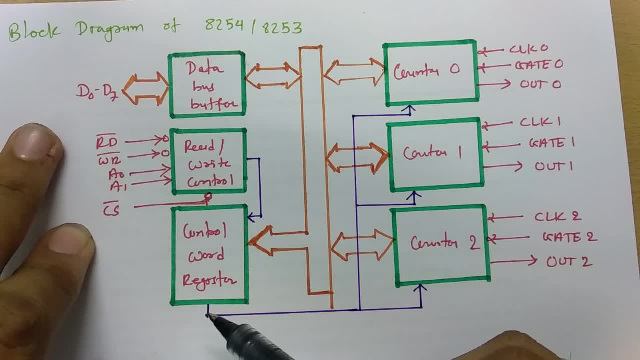 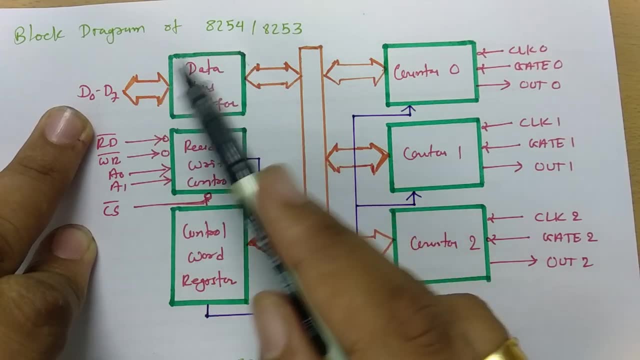 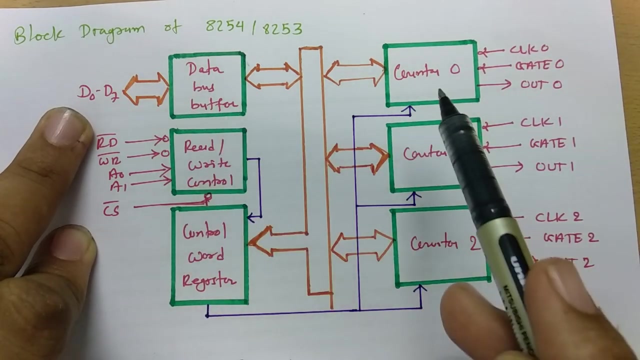 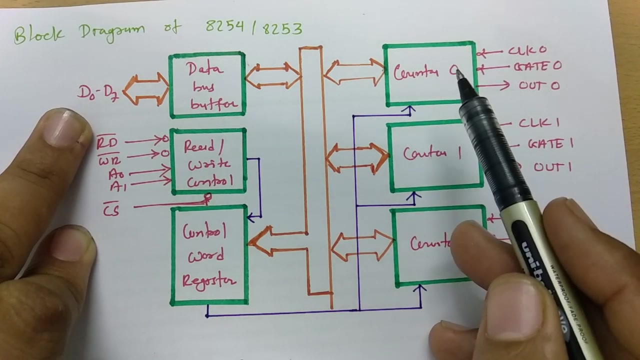 when you have control register. at that time, by exchanging data through d0 to d7, we can exchange data to this 8254. so if we place data on 8254 we can load counter data and that counting will be getting done individually like see: if counter 0 is selected, it will be counting data based on. 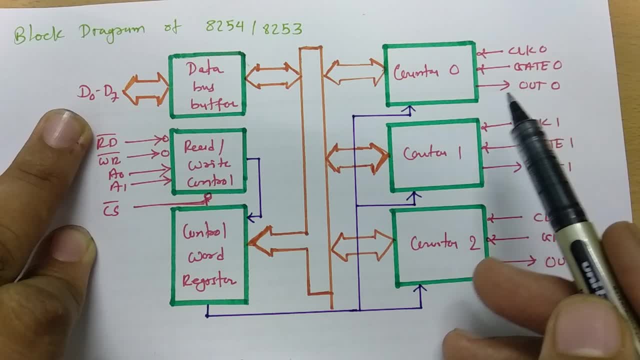 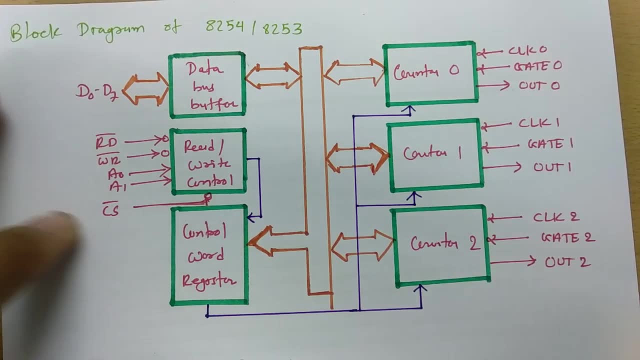 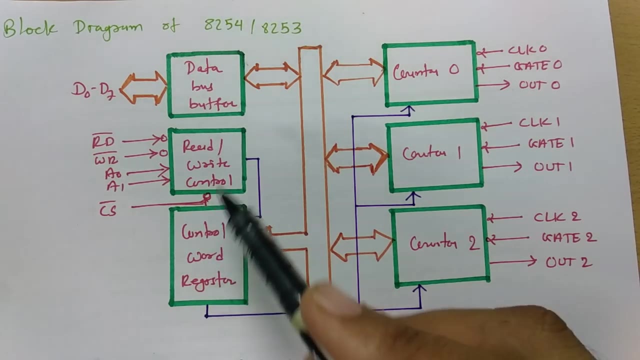 clock and gate input and it will give out counter data to this register so we can see how output over here. and similar case is there for counter 1, counter 2.. So to justify the total number of count we need to select control, register and control. 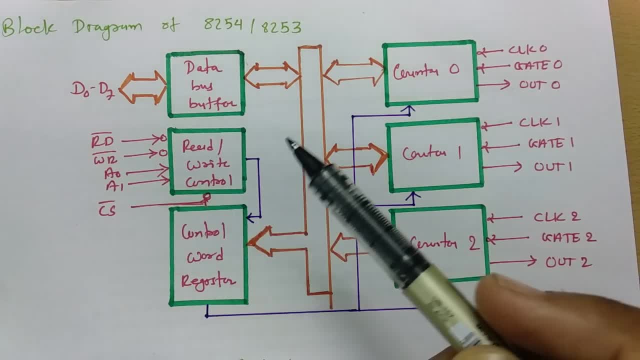 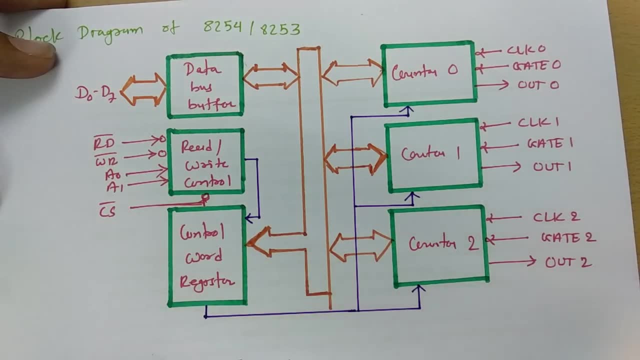 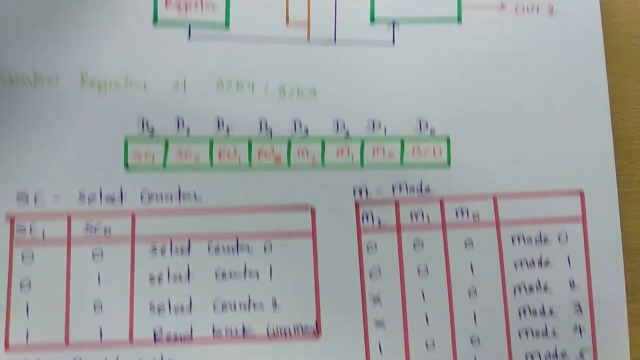 register will get selected by a0 and a1 is equals to 1: 1.. Now see if you have control register getting selected by having a0 and a1 is equals to 1: 1 you can be placing data d0 to d7 and that is assigning control register data. 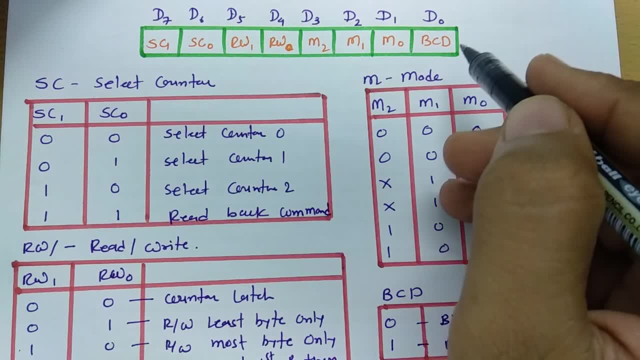 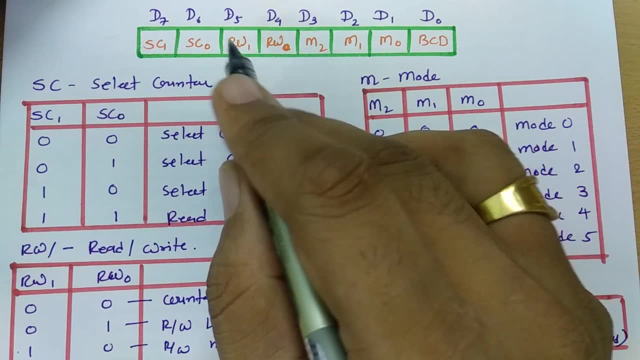 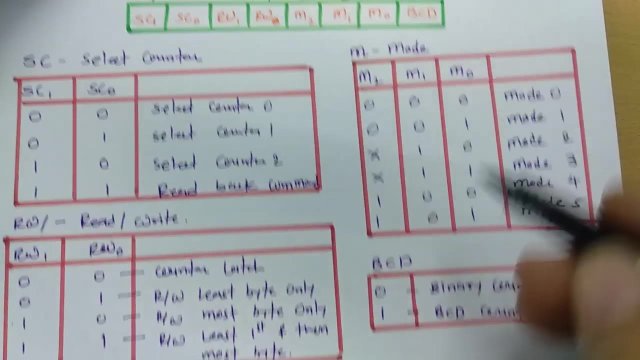 So control register from d0 to d7. that is as per BCDM0M1M2: read write 0. read write 1. SC0SC 1. Now see this first bit: d0, BCD. so that justifies if it is zero. 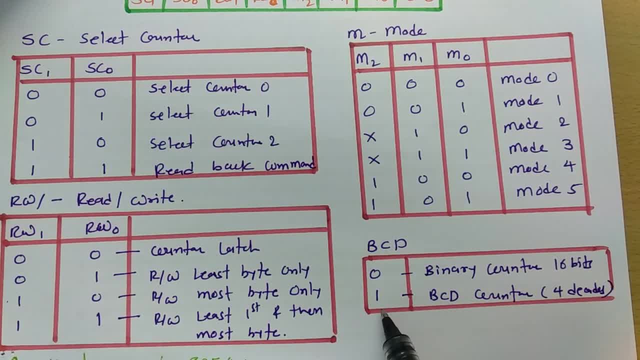 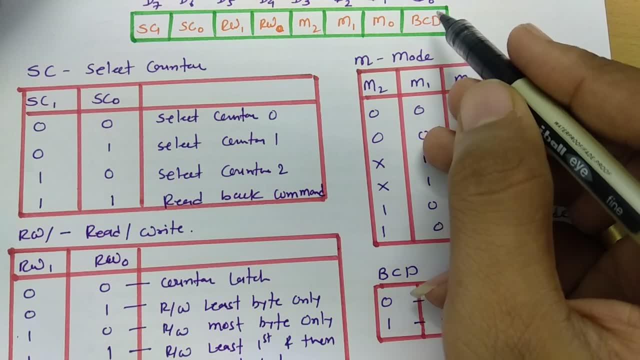 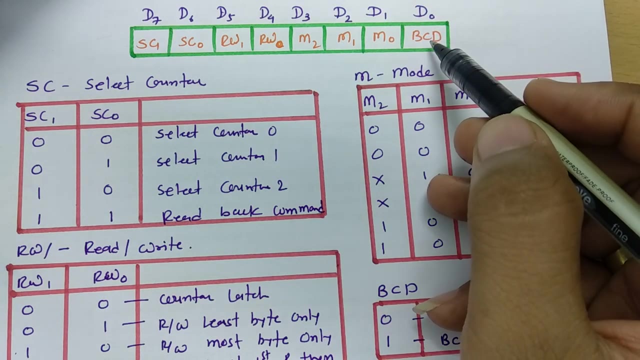 There will be binary counter of 16 bit. If it is 1,, then there will be BCD counter of 4 decades. So here this bit D0. that will justify whether this counter is binary or BCD. If it is 0, counter will be binary. 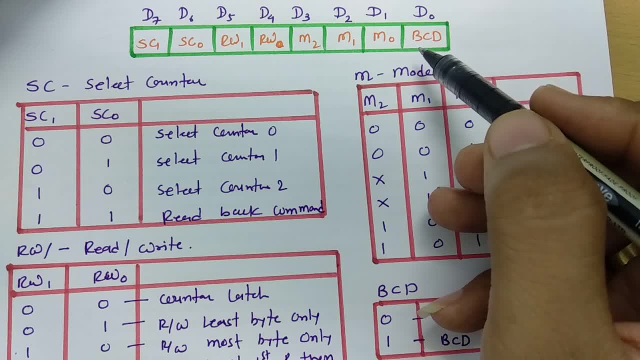 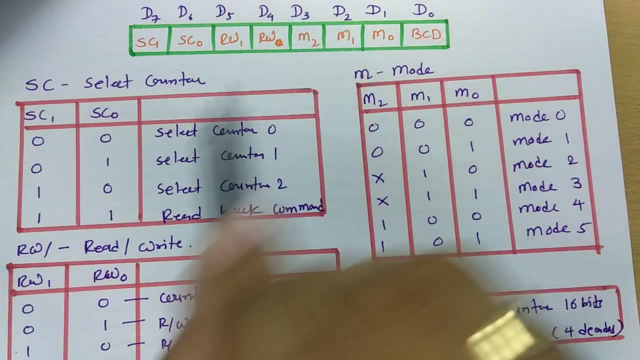 If it is 1, counter will be BCD. In binary there will be 16 bit And in BCD there will be 4 decades. It is this- M0,, M1 and M2- that will select mode of operation. 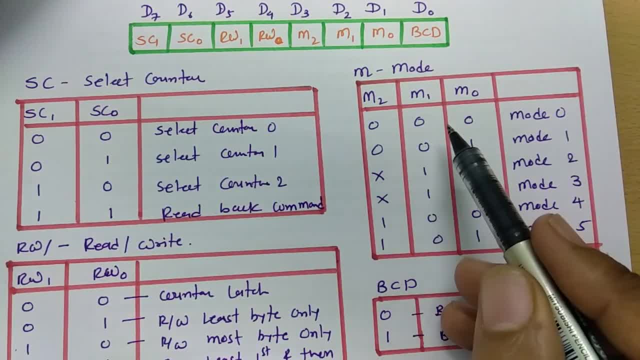 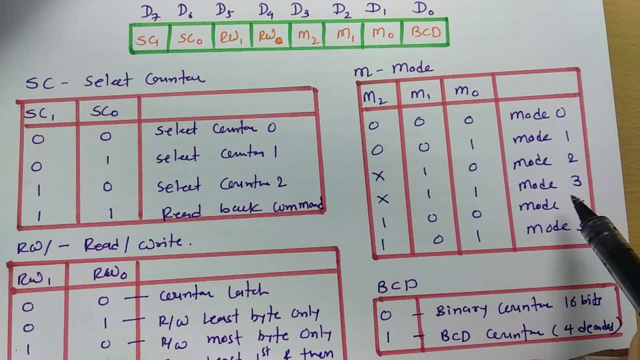 If it is 001, mode 0, 00, sorry. 000, mode 0, 001, mode 1, don't care. 10, mode 2, don't care. 11, mode 3, 100, mode 4, 101, mode 5.. 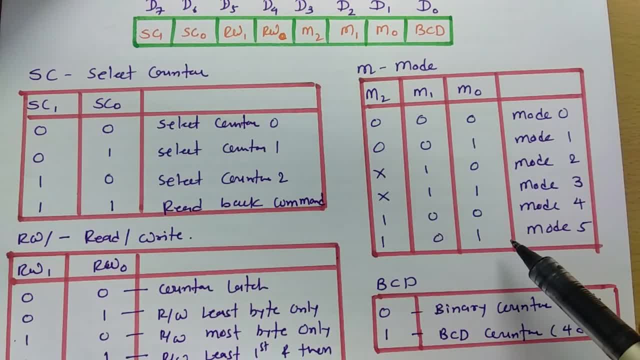 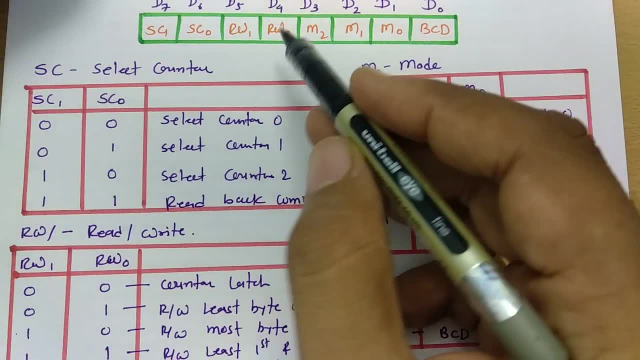 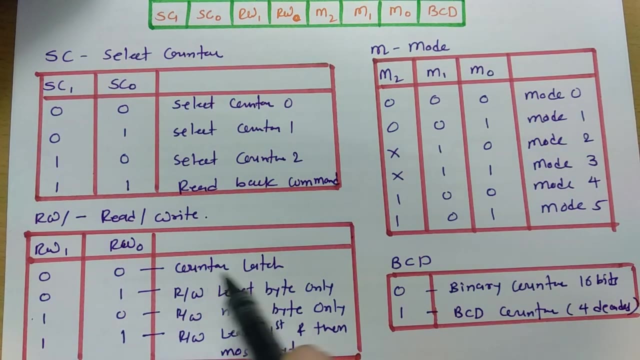 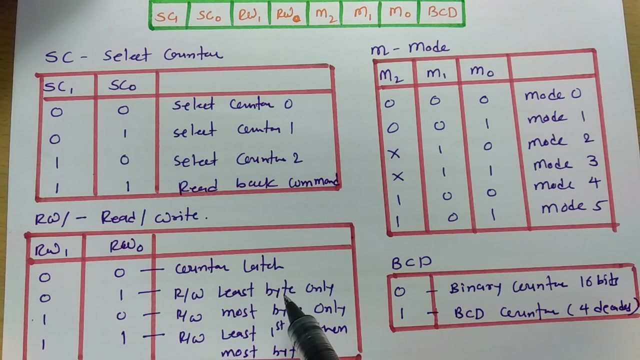 So that is how 6 different modes are there with 8254.. Now there is read write 0 and read write 1.. So if read write 0, that is 00, counter latch operation will happen. If it is 01, read write of least byte is happening. 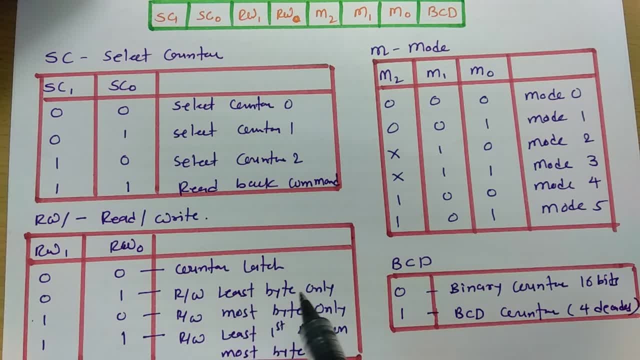 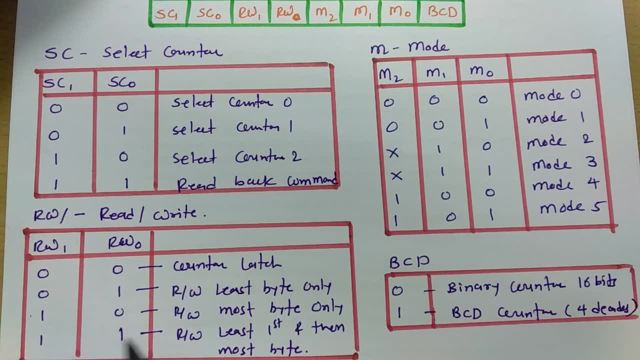 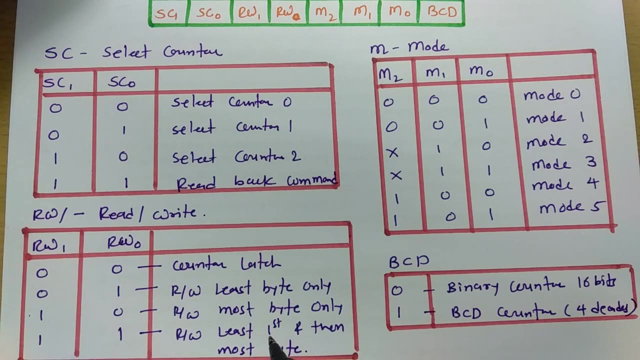 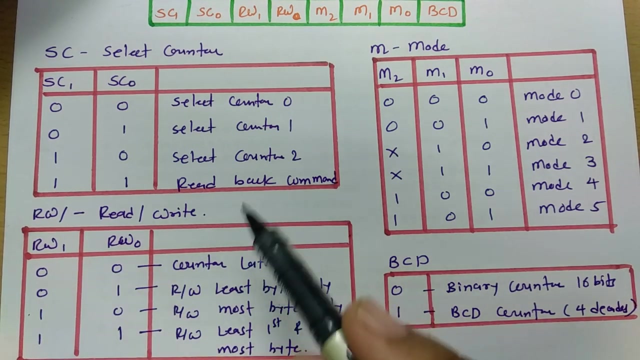 Or one can say: read, write of significant least byte is happening. If it is 10, then read write of most significant byte is happening is 11, then it will be writing or reading first significant byte and then least significant byte and then most significant byte. so that is how read, write operation. that happens so.